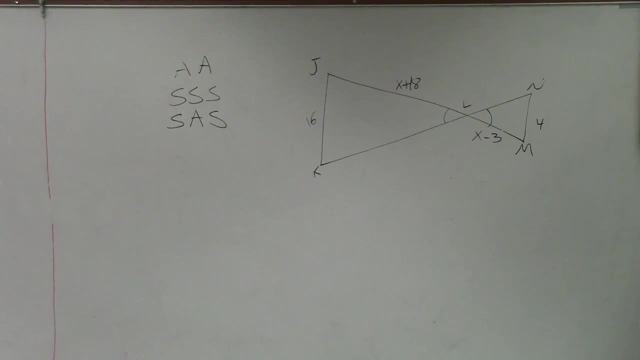 However, did they say: on this problem, did they give us: those are parallel. Which problem was this? Yeah, They said, these are parallel. OK, So that's actually so. since these are equal, though, can we now say that these are equal? 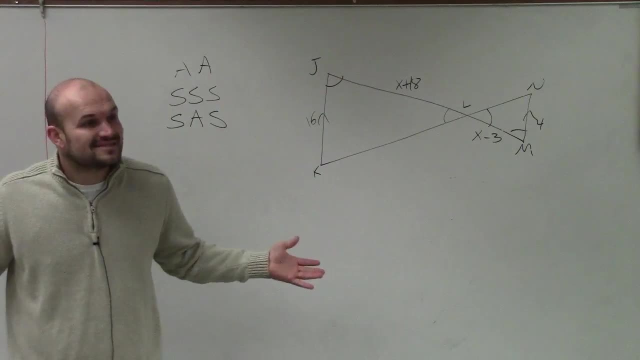 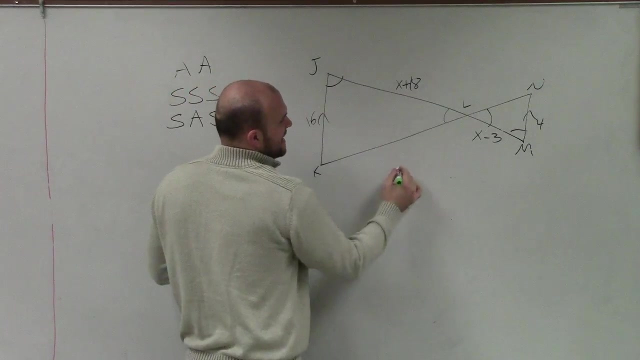 angles by alternate interior angles. Yes, Yes, So now we can use similarity. So now, since I know these are similar, I need to use proportionate sides, So I can see that x minus 3 is proportional to x plus 18, which is equal to 4 over 16.. 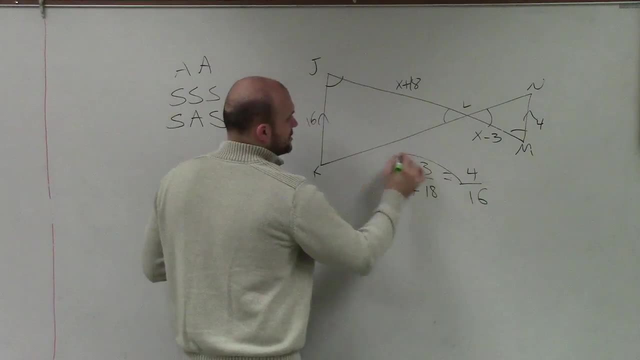 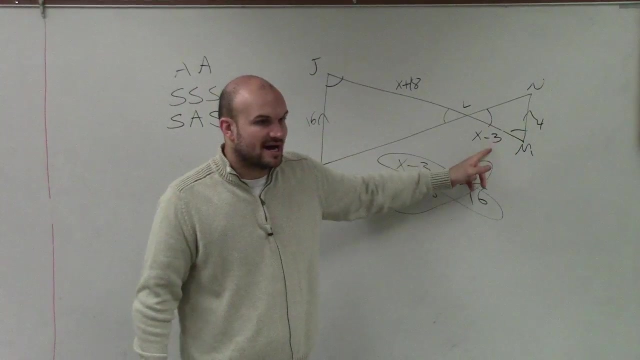 Now again, we need to cross multiply, So I use my cross products. Now again, notice guys, I only set up this proportion when I had side angle side. I knew these angles were equal, but that didn't help us out. 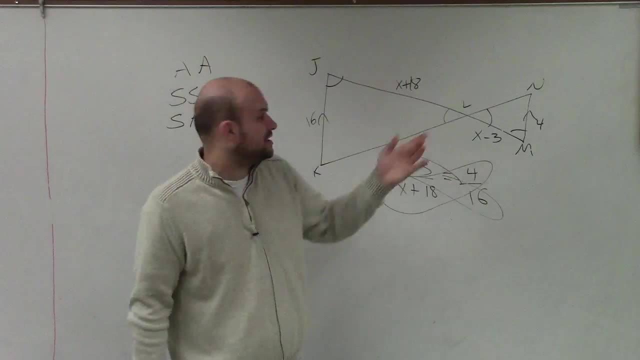 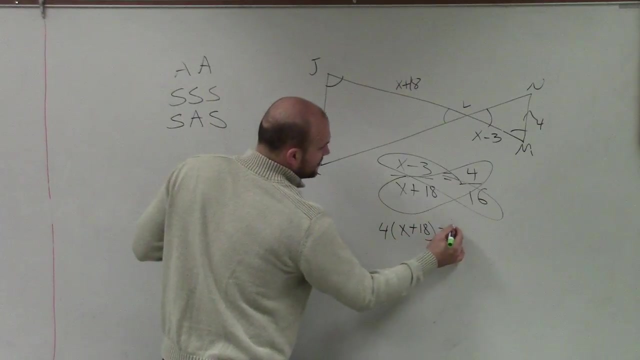 The only way I helped us out is when I had my angles in between, which I could prove by alternate interior angles. So now I apply my cross product, which is 4 times x plus 18, equals 16 times x minus 3.. 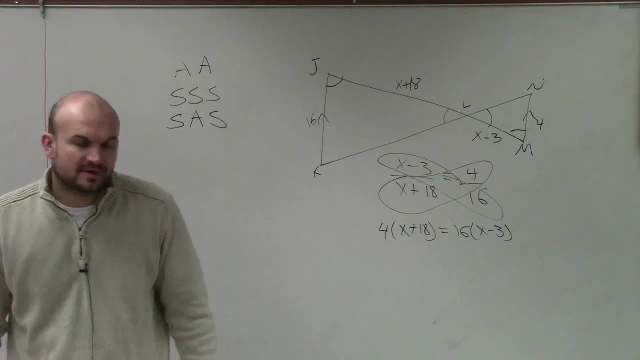 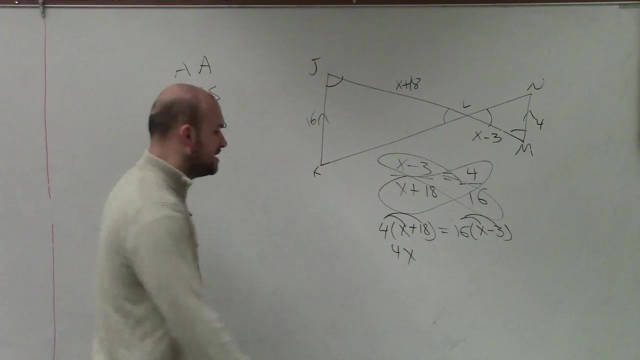 Please remember to use those parentheses when you're doing these problems. OK, Alex? Then, because the reason why is when you're applying your distributive property you're going to have a problem. If you're applying your distributive property, I have 4x minus 32, that would be 64, equals. 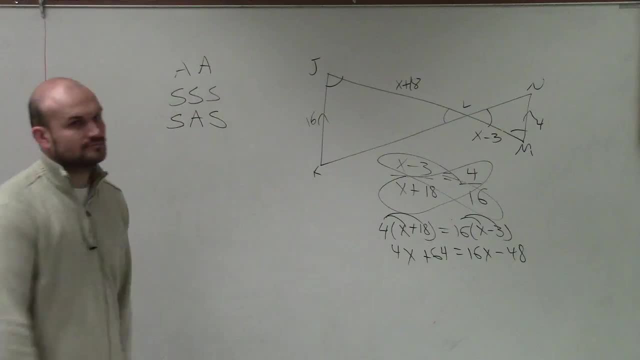 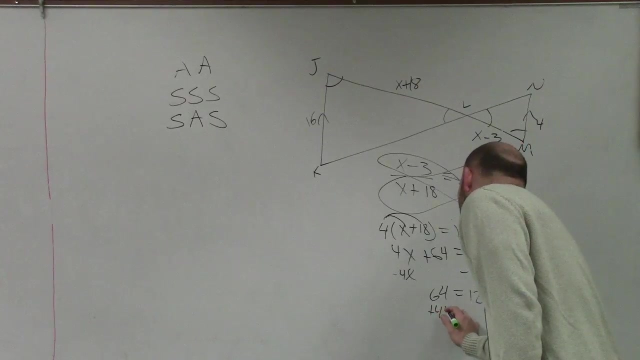 16x minus 48.. Now I go ahead and get the x's by itself. So I subtract the 4x: 64 equals 12x minus 48.. Add 48.. Add 48.. That becomes a 112.. 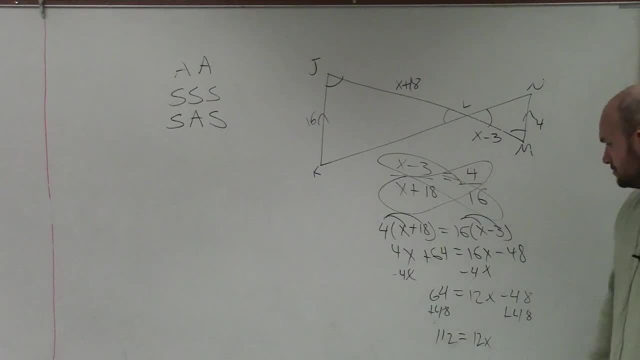 All right, Maybe I'm wrong, Huh. And then I divide by 12. Or by 10.. It would be 112 divided by 12.. How is it not 10?? Because 12 times 10, you just add the 0,.